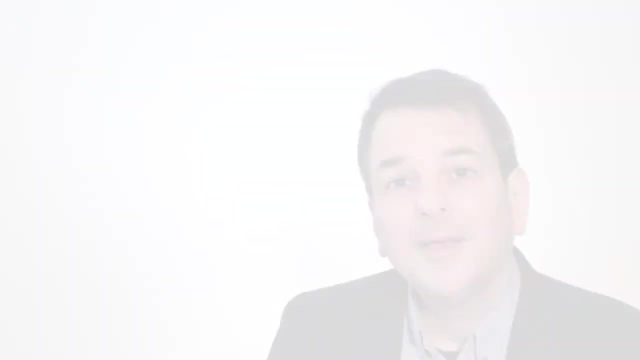 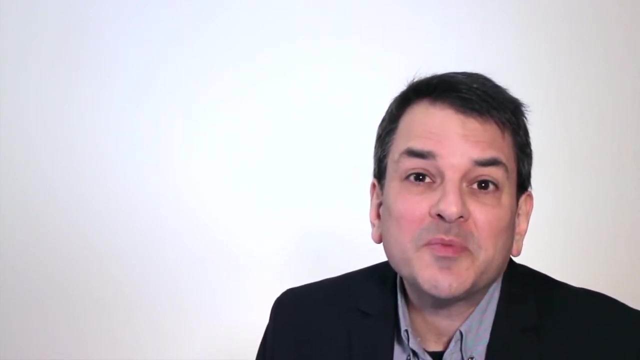 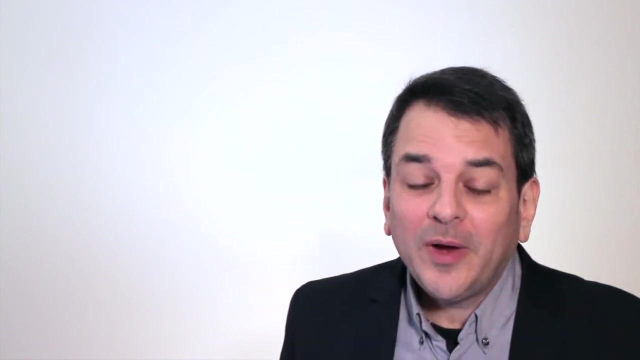 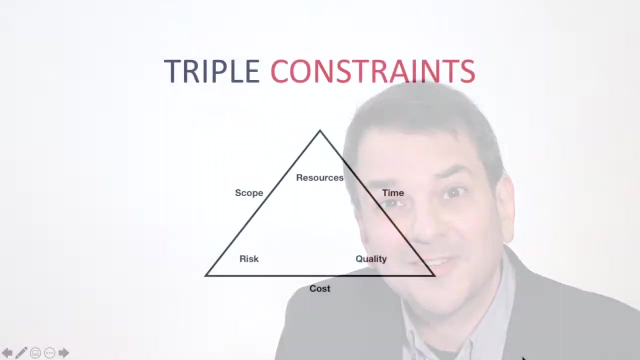 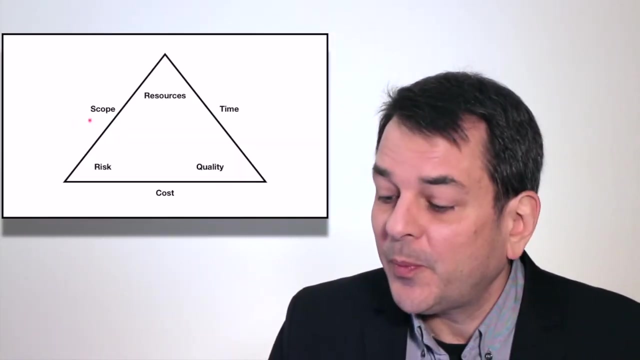 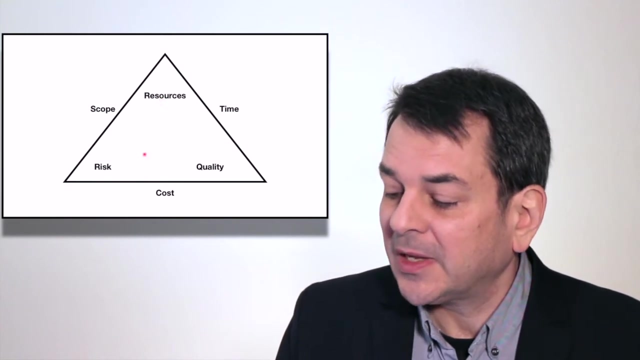 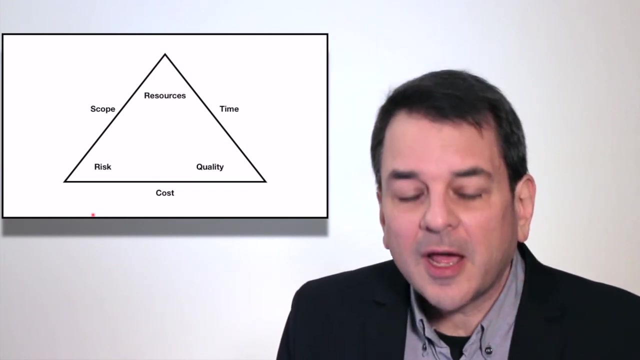 Thank you. Scope, time and cost and their relationship with quality, risk and resources. These are those common limitations, these major constraints that we all have on most of our projects, that we have to keep in balance and manage throughout the project. 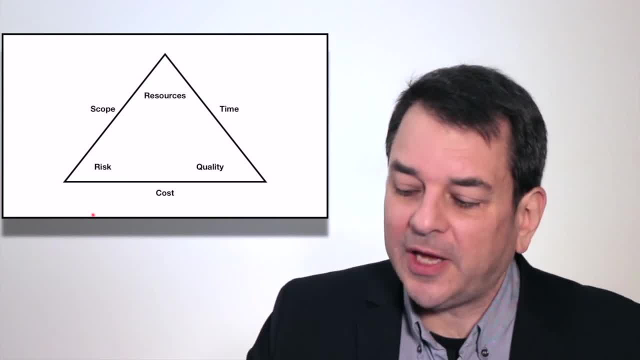 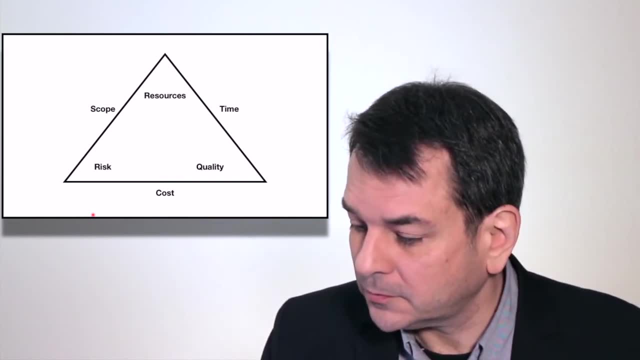 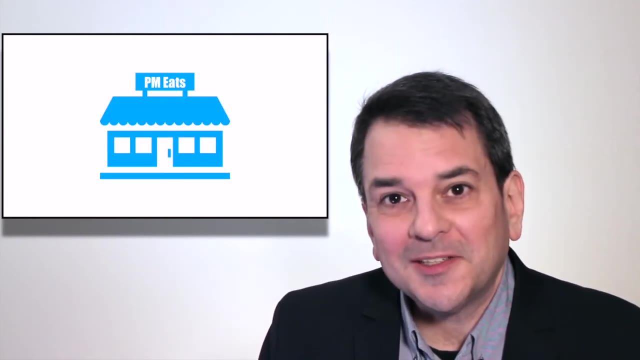 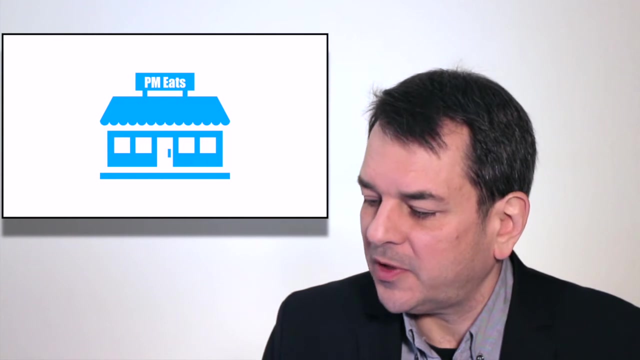 And the basic concept here is that any change to any one of these constraints has a potential impact on any or all of the other ones. So let's say we own a restaurant- PM Eats- and we want to increase revenue, So we come up with the idea for an interior renovation project. We're going to modernize the kitchen, we're going to expand the dining room and we do some analysis and research And it suggests that we could expect a $30,000.. $30,000 revenue increase within the first year of completing this renovation project. 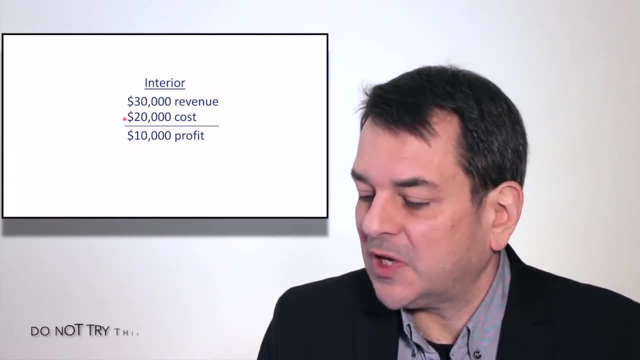 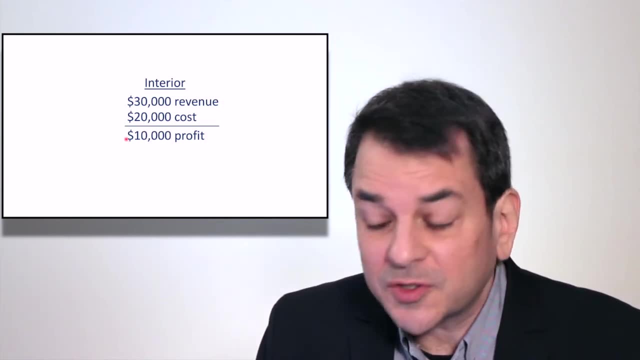 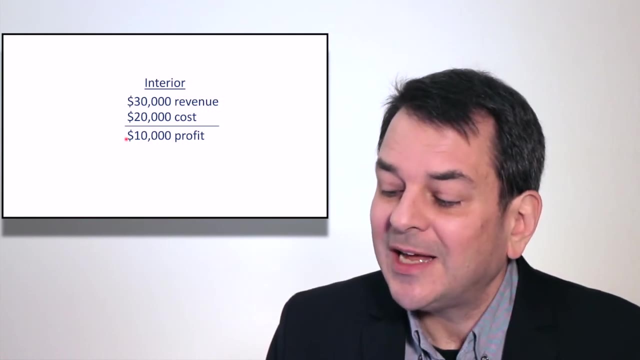 And our cost estimates show it's going to cost about $20,000 to do the renovation. That leaves us a very nice profit of $10,000.. So from a financial standpoint this return on investment looks pretty good. We're excited about this project. 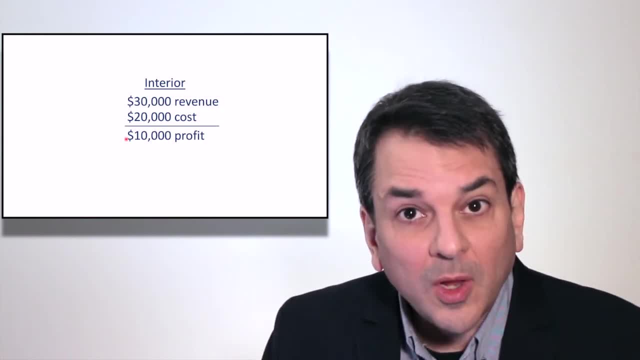 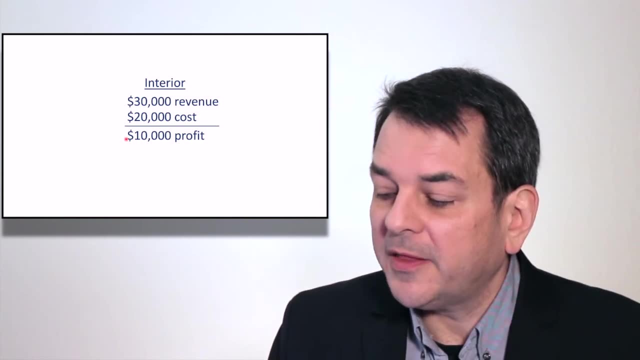 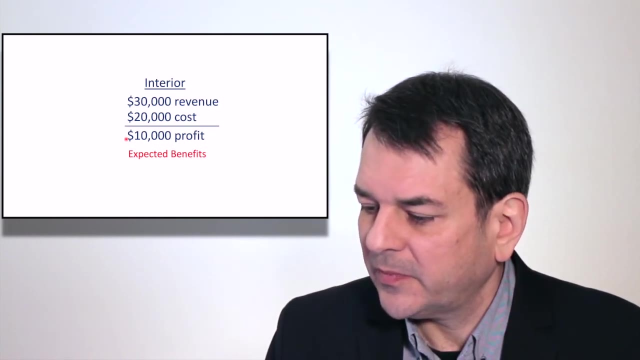 And this $10,000 becomes our target, our goal that we're shooting for. It's the financial justification for why we're doing this project. We call this our expected benefits And let's clarify what's in scope and out of scope for this project. 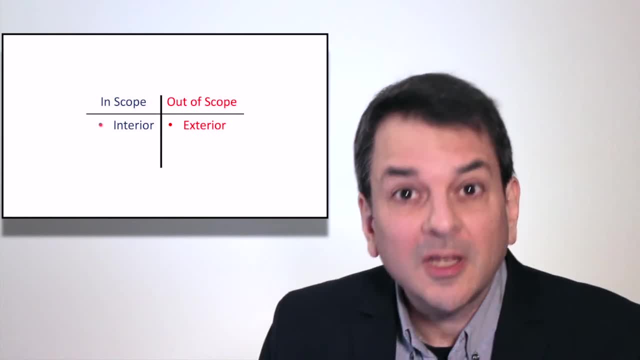 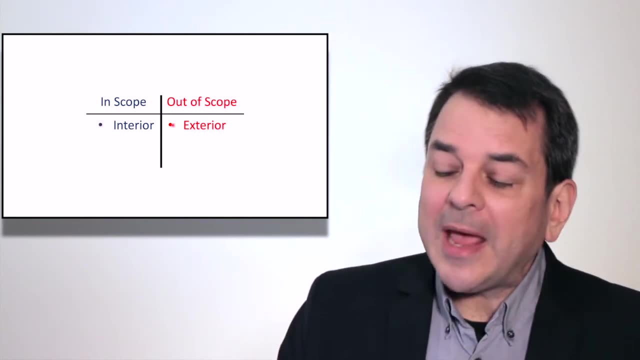 So we committed to that. it's only about the interior renovation. We're going to modernize the kitchen, expand the dining room, make improvements to the restroom. We considered painting and signage on the exterior, But we decided: no, that's something else. 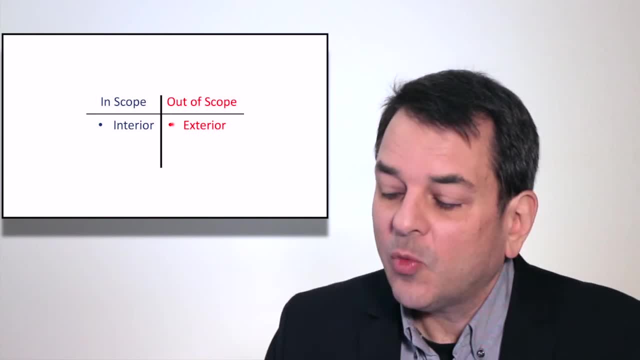 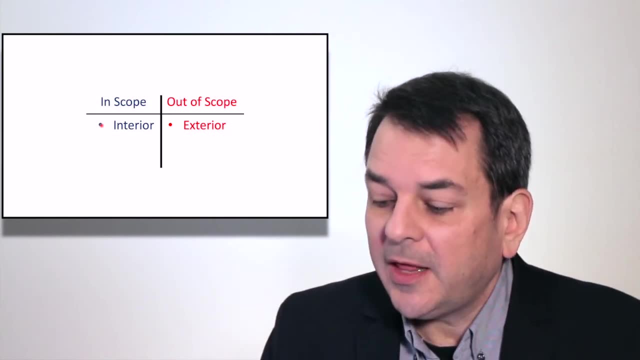 We're not going to do that now. We might revisit that later, But for now we're just going to focus on the interior. So we collect our requirements for the interior renovation project And that helps define our scope of work for the project. 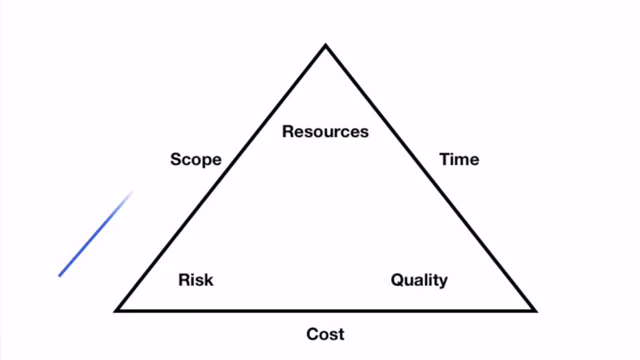 So now we have an idea of our scope of work, We figure out, well, what's a reasonable timeline, What's a reasonable budget? Is the $20,000 enough? And in order to do that, we would be making trade-offs with quality, which fixtures we have in the kitchen? 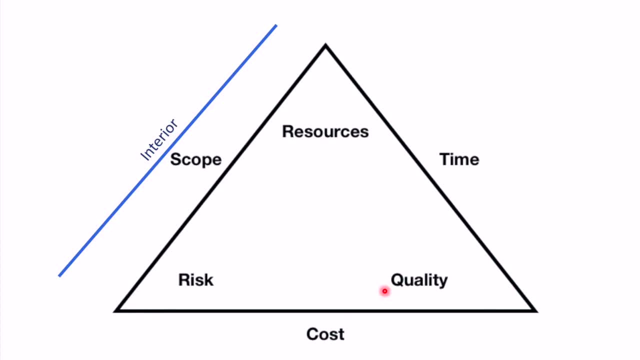 what quality management efforts, the quality checks, the quality testing We're going to build into our processes while we're managing the project. We make similar trade-offs with risk management: How much risk exists in this project And what is a reasonable amount of effort to do to manage that risk. 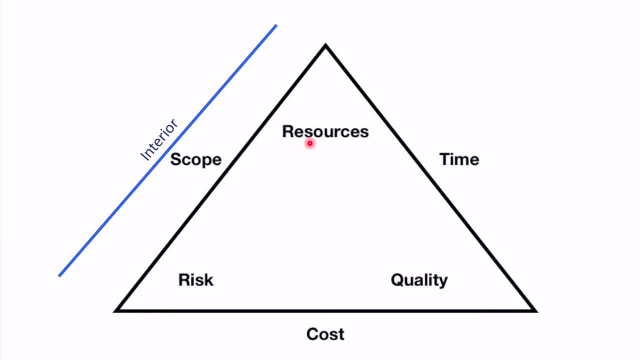 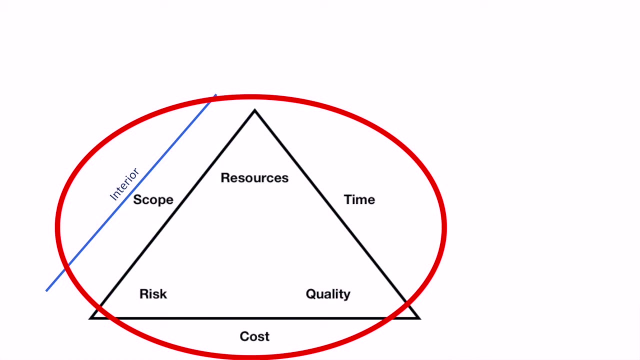 Trade-offs with resources. What resources are available to us? What human resources are we going to hire in order to do the work? What supplies, what equipment do we need? So we find a nice balance between all these, based on the information we have at this point in time. 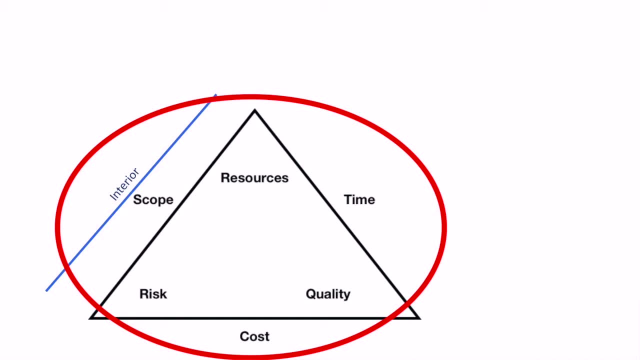 And we also want to make sure it's in balance with our ultimate goal of this $10,000 profit. So, based on the information we have at this point in time, at least on paper, everything looks in line with each other. So we make sure that we have a balanced budget. 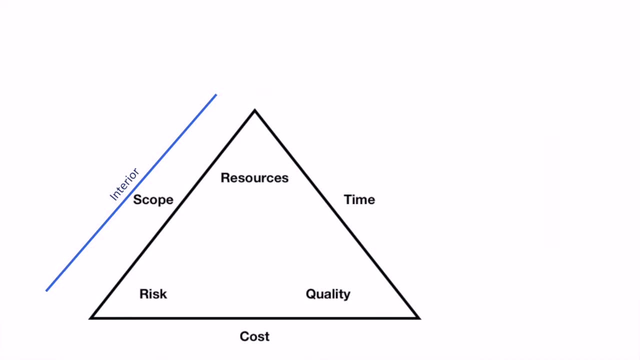 We move forward, we do some planning and we start doing the work, And then one day our boss shows up and says: hey, let's do that exterior. after all, It makes sense to do it all together. Let's just do it. 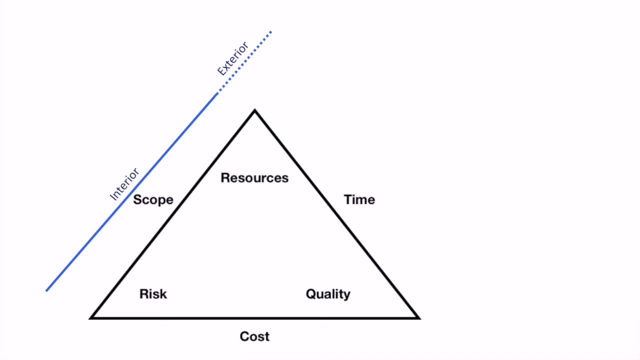 If we drop everything and just do it because our boss asked us to do it, we're going to be in trouble. We're going to run out of time, We're going to run out of money Or, in order to stay on schedule and on budget, we're going to cut quality so much. 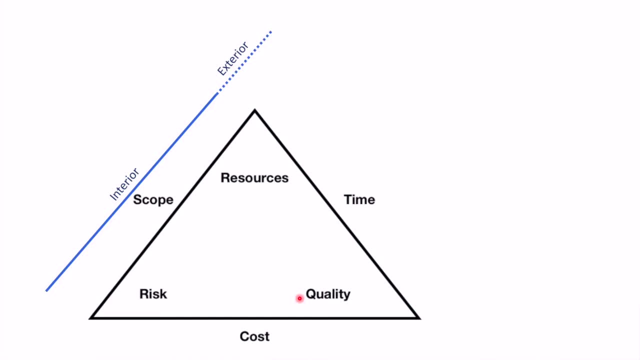 we're just going to have a crappy renovation. We're going to have a crappy renovation job that's not going to get this $30,000 in revenue, in this $10,000 profit that we're shooting for. So what we do is we pause and before we commit to this exterior part of the project, 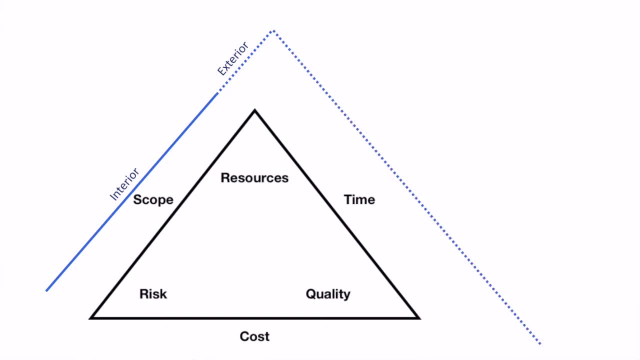 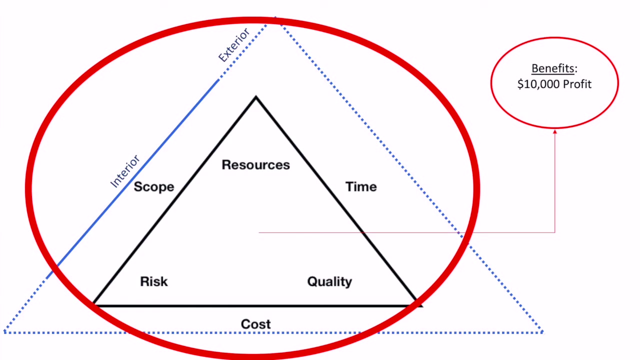 we evaluate. well, what does this mean to the timeline? What is a reasonable budget to finish this? What are the new trade-offs with quality, with risk, with resources, And is it still in balance? What is our goal of making a profit on this?